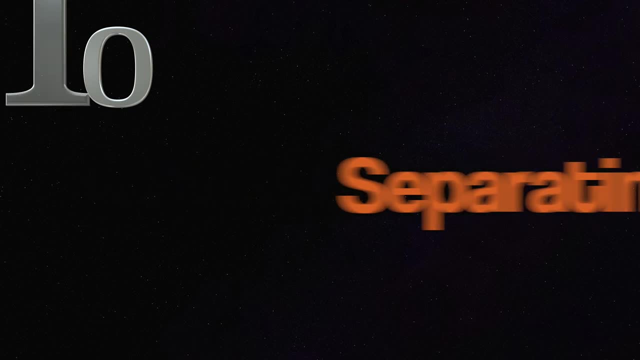 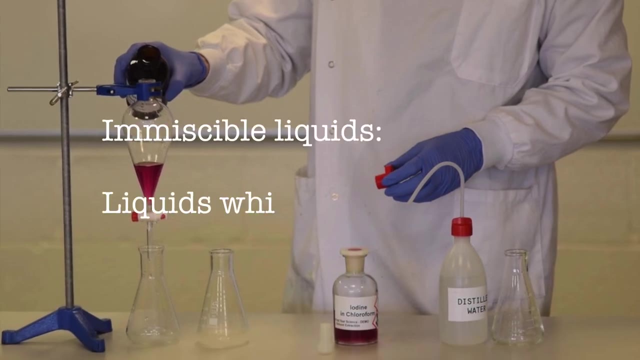 10. Separating Funnel. Separating funnel is used to separate two immiscible liquids with different densities. Immiscible liquids are those which won't stay mixed to give a single phase. Oil and water can be easily separated using this technique. 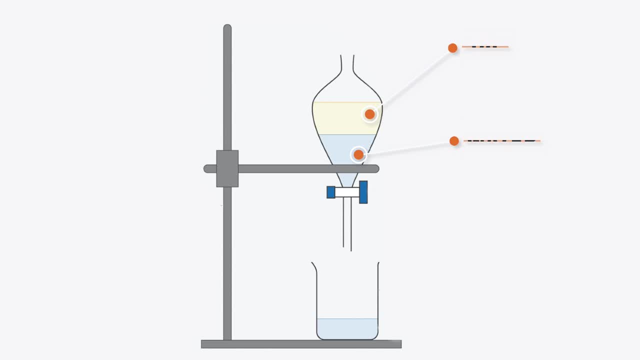 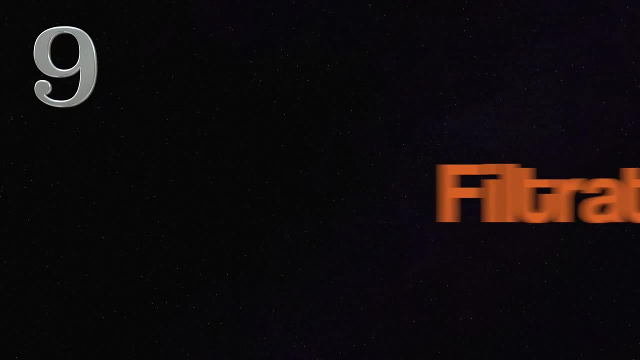 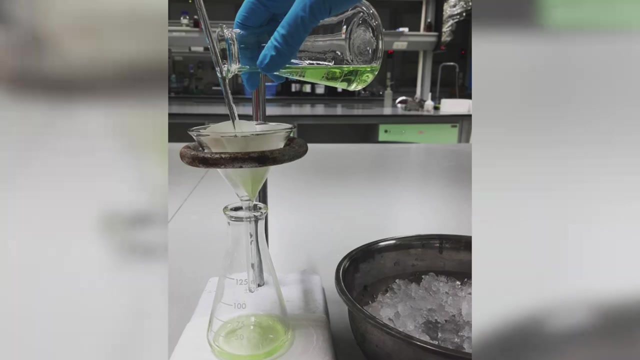 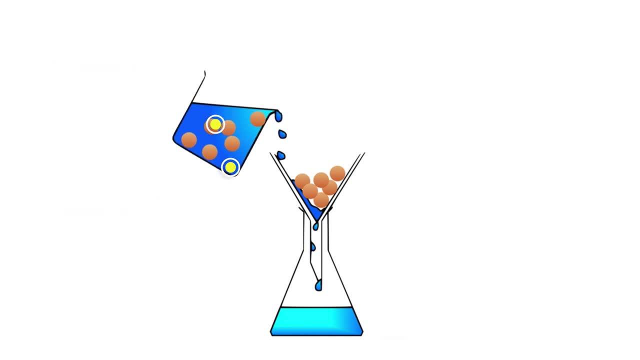 When a mixture of sand and water is filtered, the sand stays behind in the filter paper and it becomes the residue. The water passes through the filter paper and it becomes the filtrate. Various filtering agents can be used, like filtering paper or other materials. 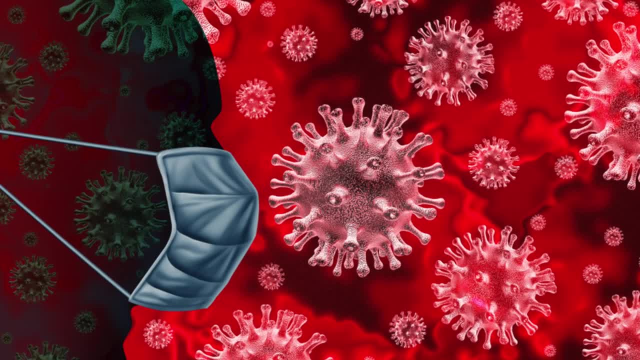 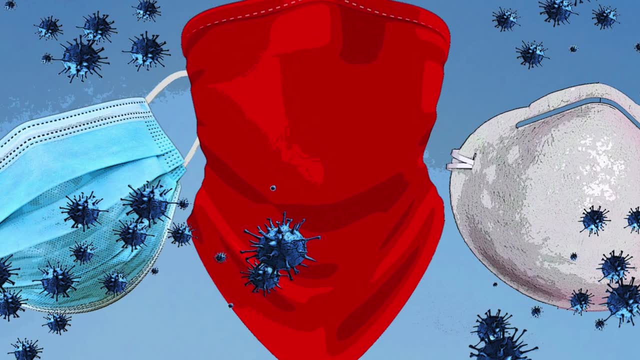 One of the very important filtering material these days is a mask. By wearing a proper mask, coronaviruses will be filtered and stay outside of the mask. Only the clean air goes through the mask. If you want to find out more about filtration process, 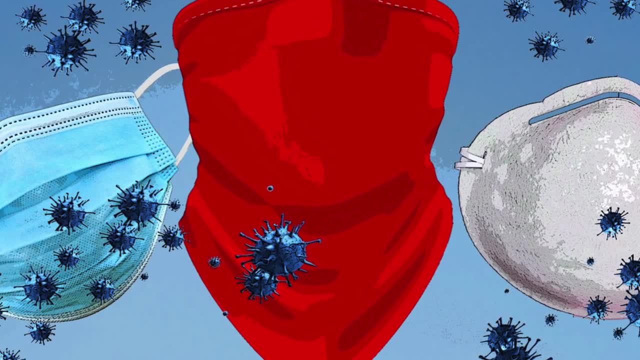 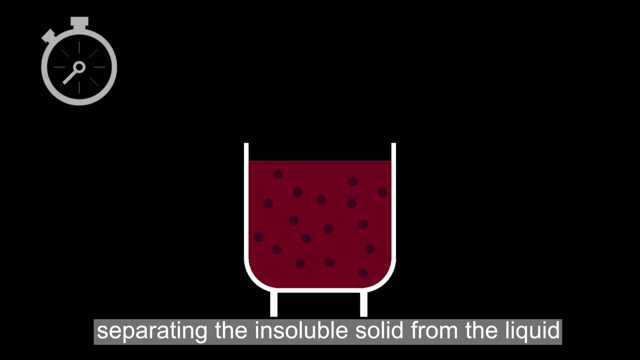 you can watch my previous video called filtration. Please click the link above. 8. Sedimentation: Sedimentation is the process of separating the insoluble solid from the liquid. Heavier particles present in liquid normally settle down at the bottom of the container. 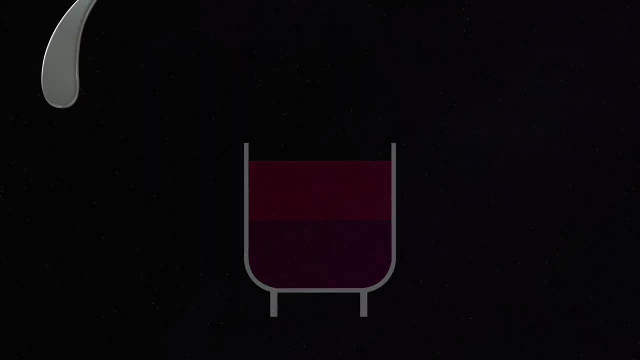 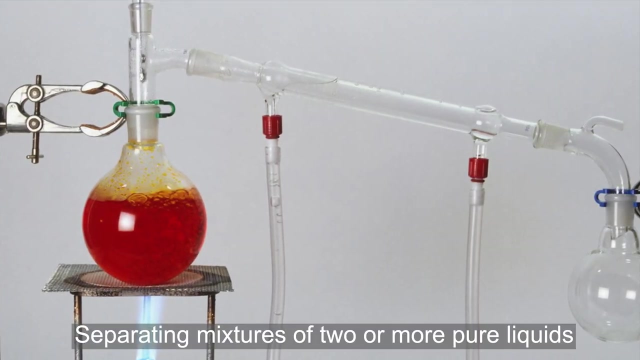 The process, however, takes some amount of time. 7. Distillation: When mixtures consist of two or more pure liquids, distillation method can be used. In distillation procedure, the round bottom flask contains the liquid mixture, which must be heated. 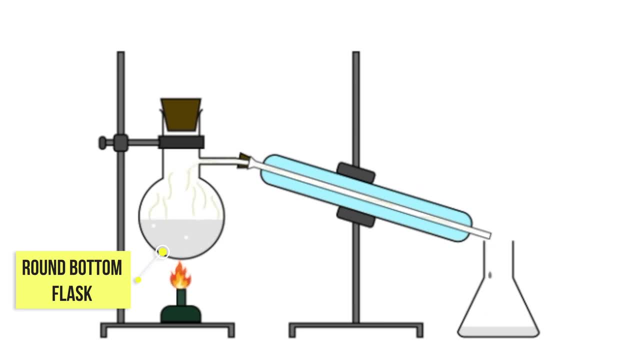 to a vigorous boil. The component with the lower boiling point will change into a vapor. The vapor moves through a condenser. The vapor condenses and is collected in a liquid Distillation method. is collected in a liquid state. The other liquid component remains in the round bottom flask. 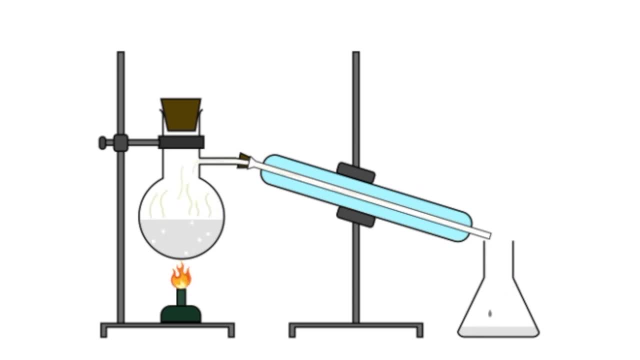 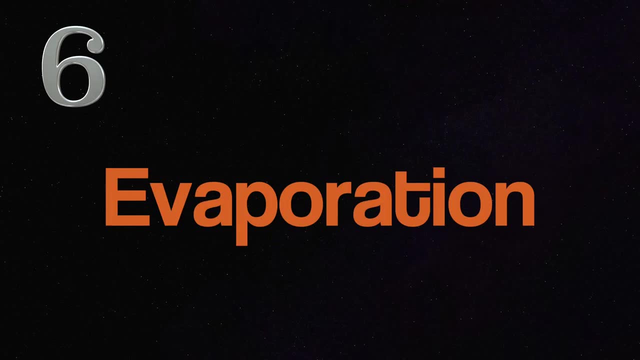 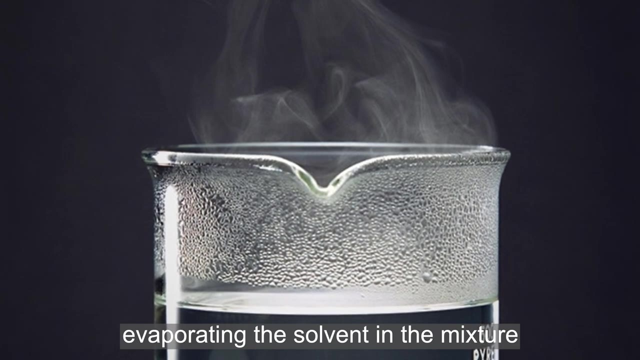 If you want to find out more about distillation, you can also watch my previous video called distillation. Please click the link above 6. Evaporation: Evaporation is a separation method that involves evaporating the solvent in the mixture. In this method, the solution is heated until the organic solvent evaporates. 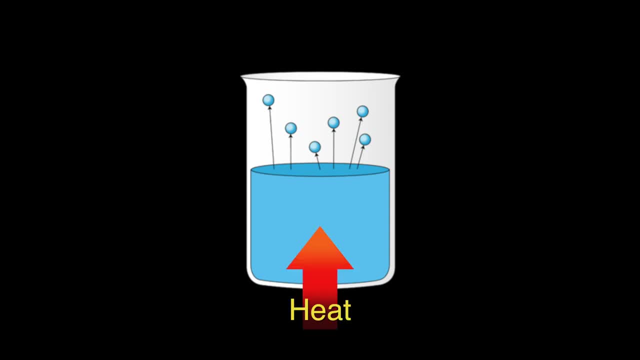 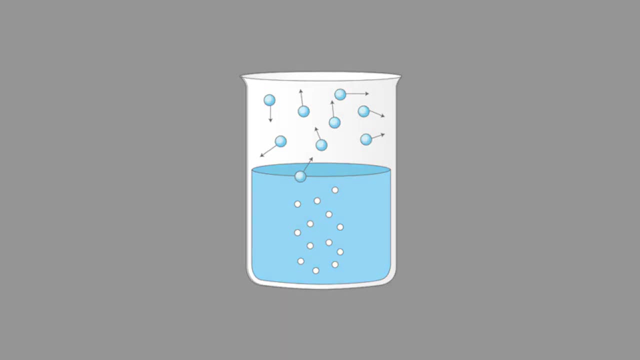 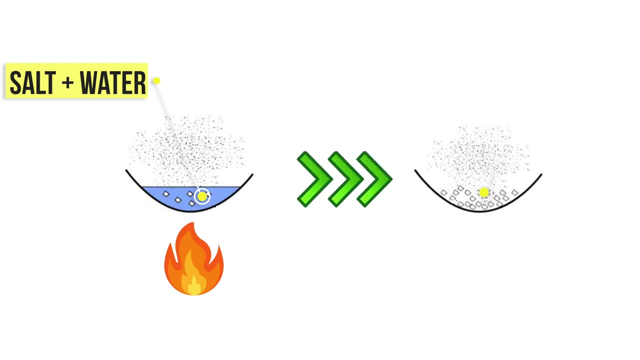 It turns into gas and mostly leaves behind the solid residue. Once the liquid is completely evaporated, the solid is all that is left behind. An example of this is a salt and water mixture, where the water can be evaporated in order to leave the salt behind. Did you know that most of the salt that we use 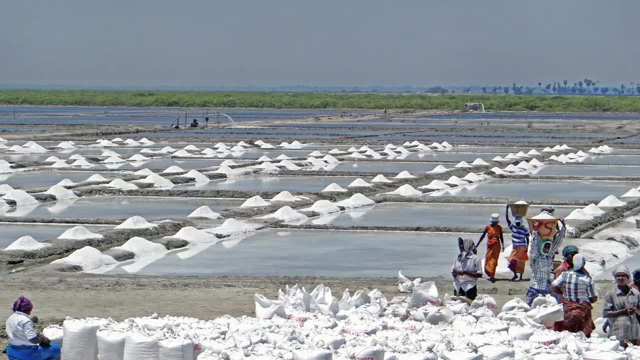 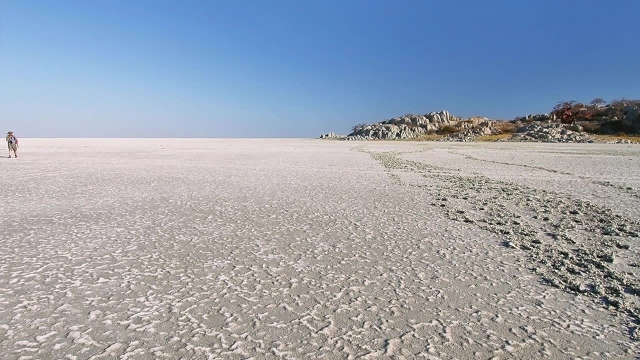 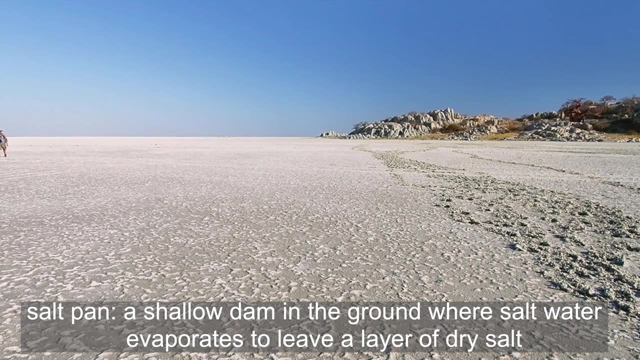 come from South Africa. Well, South Africa gets its salt from inland salt pans, coastal salt pans and salt water by using the evaporation process. A salt pan is a shallow dam in the ground where salt water evaporates to leave a layer of dry salt. 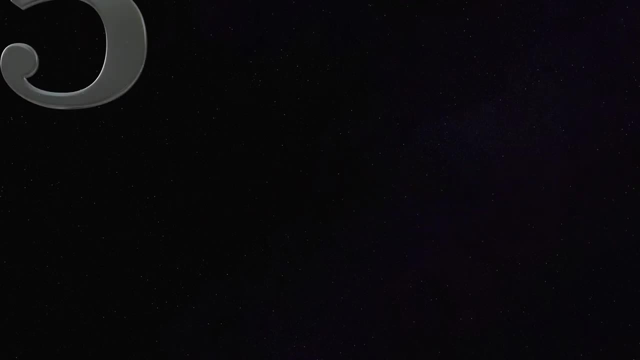 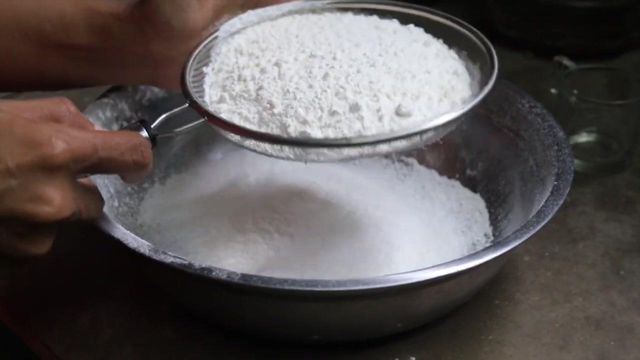 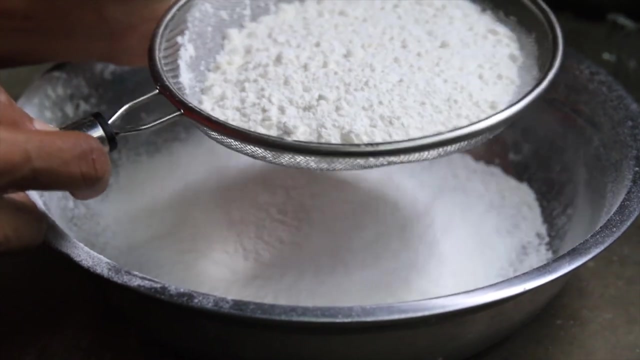 5. Sieving: Sieving is used to separate mixtures that contain substances mostly of different sizes. The mixture is passed through the pores of the sieve. The smaller substances pass through easily, while the bigger components of the mixture are retained. 4. Evaporation: 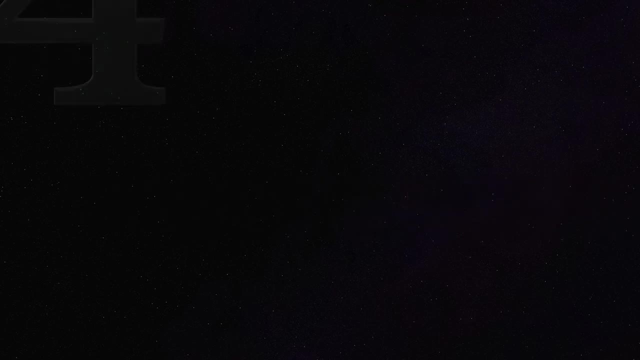 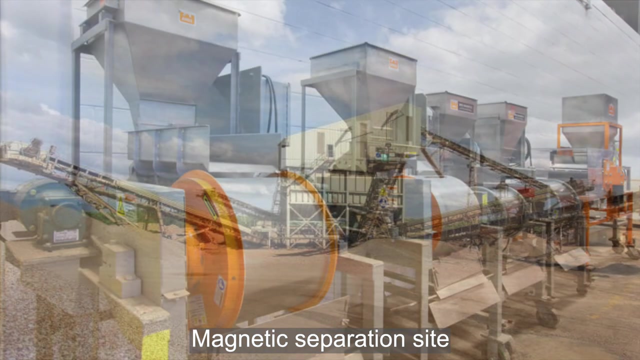 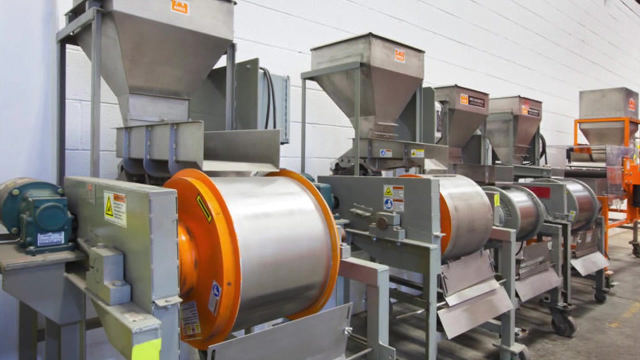 4. Magnetic separation. When one substance in the mixture has some magnetic properties, then this method can be quite useful. Strong magnets are commonly used to separate magnetic elements. Well, how does magnetic separation work? For example, mineral ore that contains two compounds. 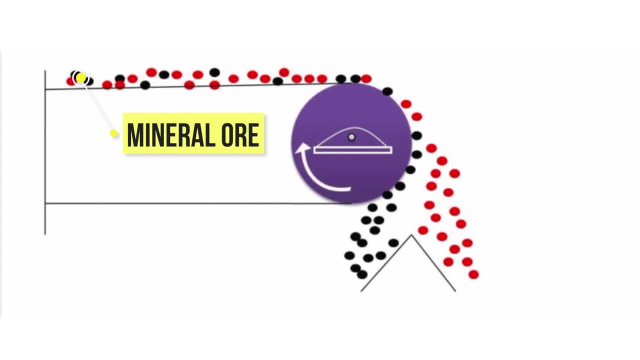 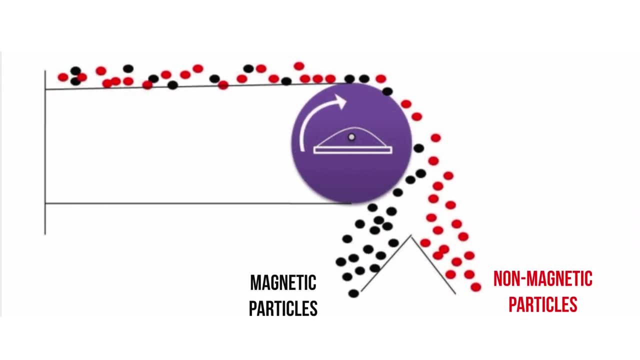 one magnetic and the other non-magnetic, can be separated using this method. The ore grains are fed onto a revolving belt. The roller at the end of the belt is magnetic. This means that all the magnetic grains in the ore will stick to the belt when it goes around the roller. 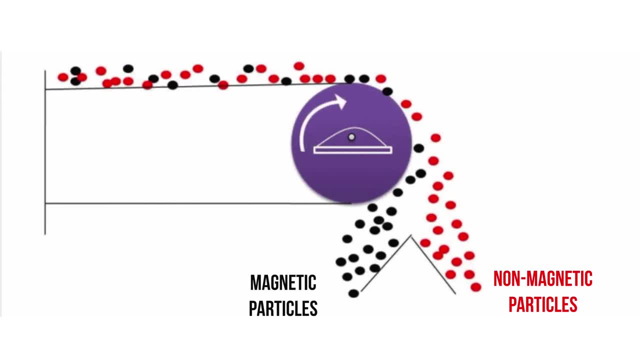 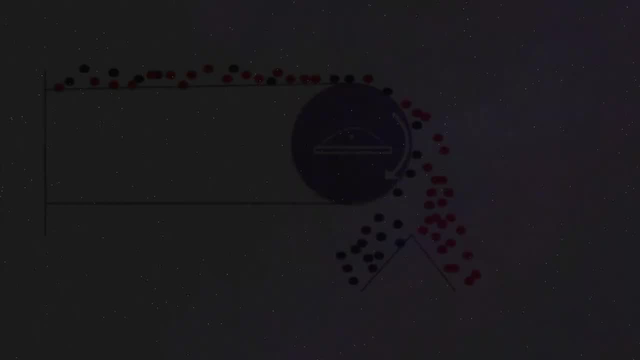 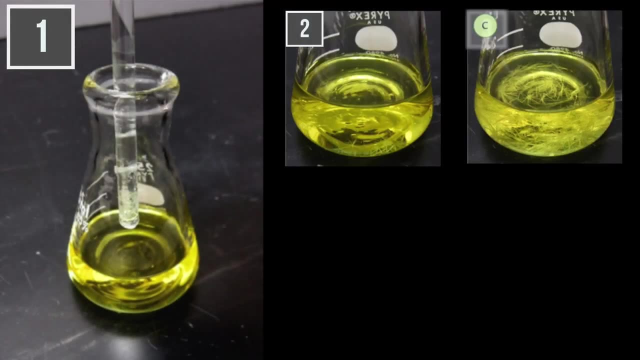 while the non-magnetic grains will fall off the end. As soon as the magnetic grains move past the magnetic roller, they will also fall down. 3. Crystallization: Crystallization is an evaporating technique that works to form crystals of the solute. 2. Chromatography: 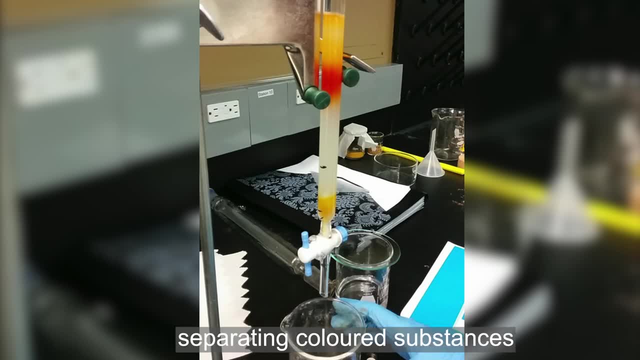 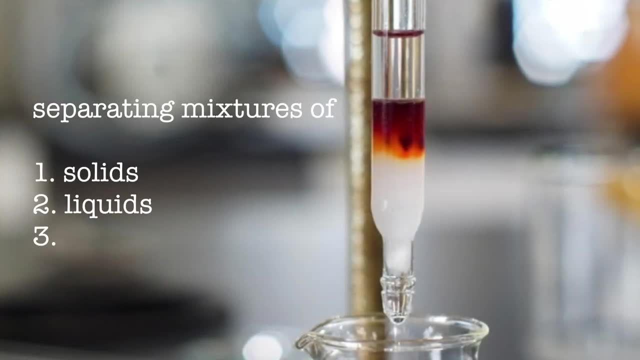 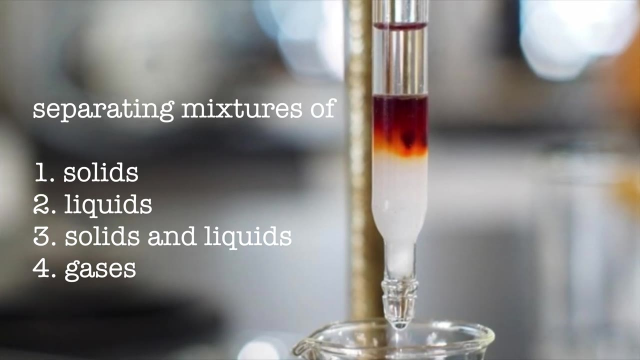 Chromatography is a method for separating colored substances into individual pigments. It is quite versatile: to separate mixtures of solids or of liquids, or mixtures of solids and liquids combined, or mixtures of gases in the case of gas chromatography. 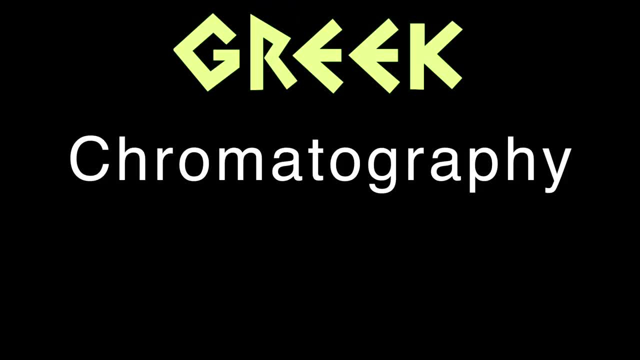 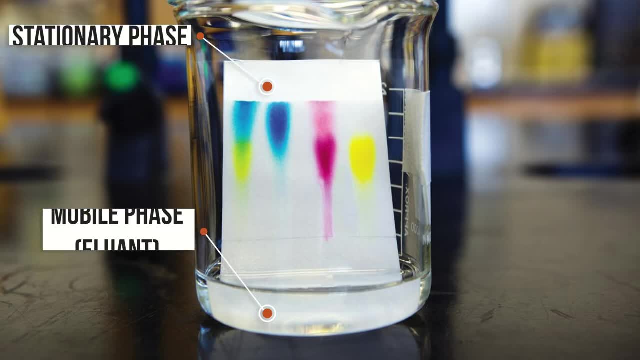 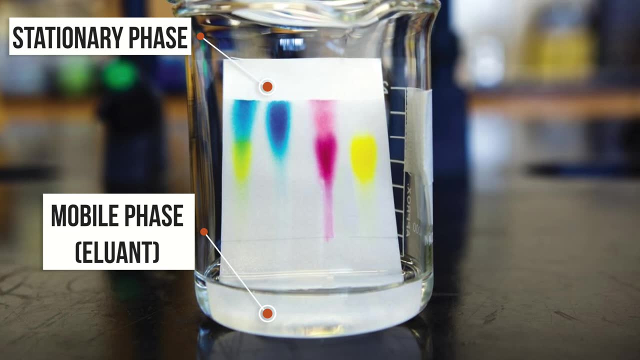 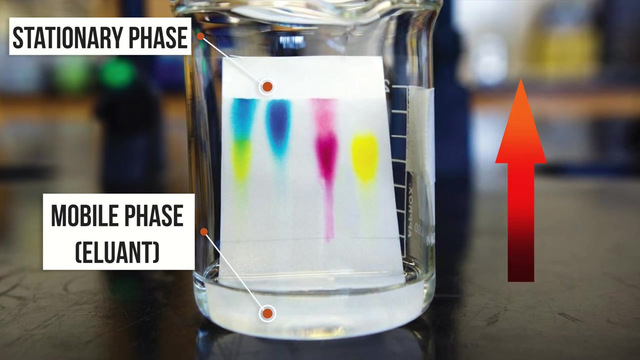 The name chromatography comes from the Greek word chroma, meaning color, graph, meaning to write. The two elements of chromatography are the stationary phase and the mobile phase. The mixture is placed on the stationary phase. The mobile phase. a mixture of solvents or eluent passes over the mixture and continues to pass through the 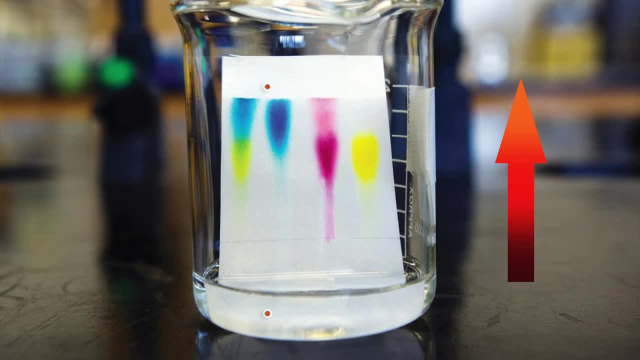 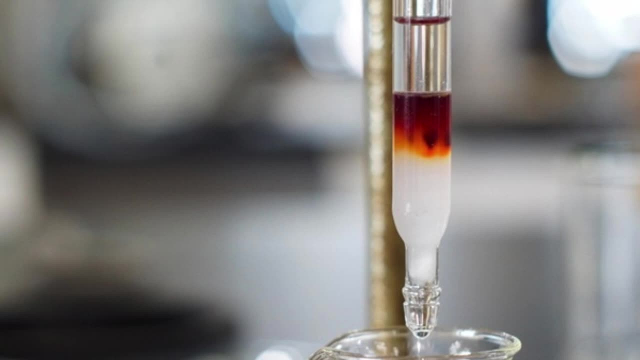 stationary phase carrying along the components of the mixture. Why are the different pigments carried at different speeds? Why are the different pigments carried at different speeds? Well, pigments migrate at different speeds because of differences in their properties. Large pigment particles. 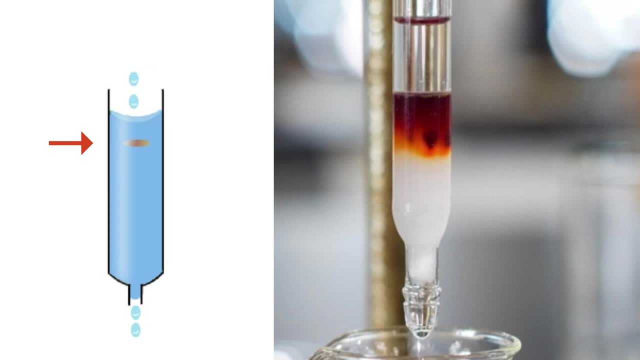 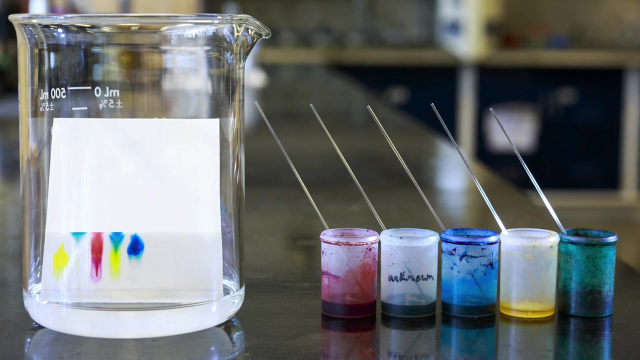 tend to move slowly. Furthermore, particles that dissolve well in the liquid will tend to stay in the liquid and be carried to the top quickly, while particles that bind well to the paper will tend to move slowly. Paper chromatography is often used when the dissolved substances are colored, such as inks, food colorings and plant dyes. 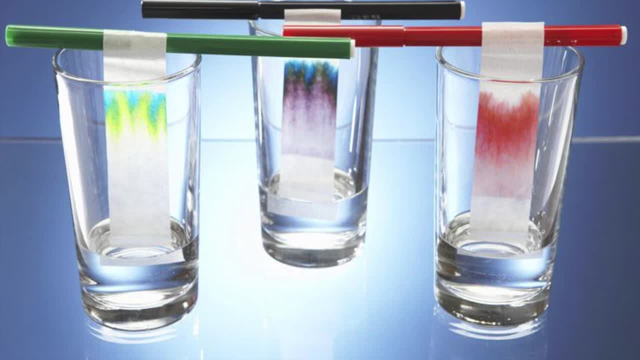 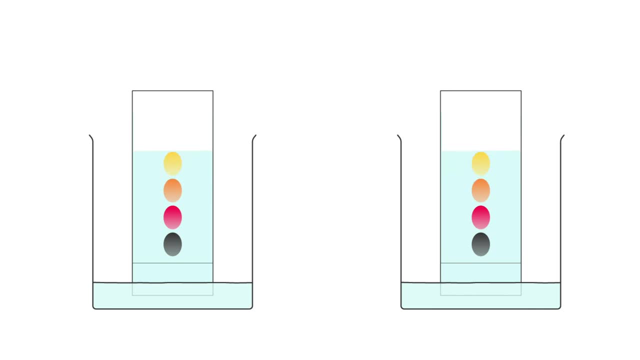 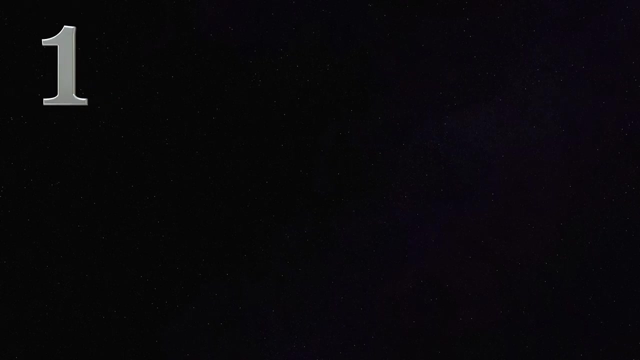 A pure substance will only produce one spot on the chromatogram. using paper chromatography, Two substances will be the same if they produce the same color on the spot and their spots travel the same distance up the paper. Number one: centrifuge. In some cases, where the solid particles 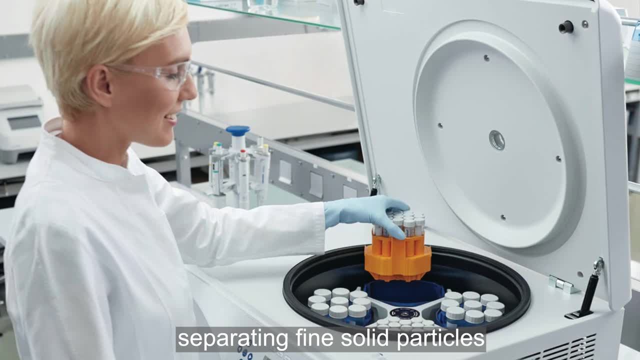 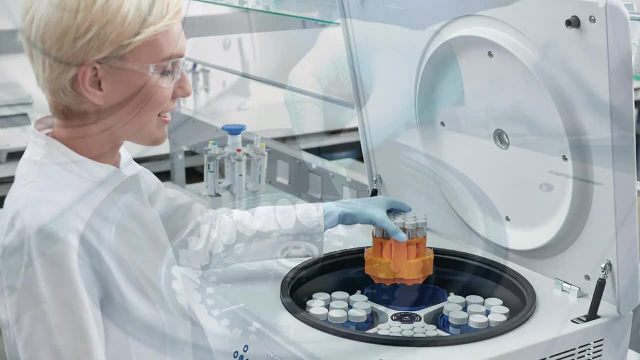 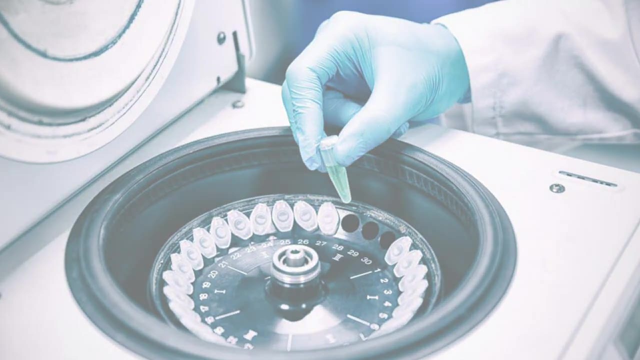 are too fine to be separated with a filter, a centrifuge can be used. Centrifuges are devices that spin at very high speeds. These high speeds allow the solid particles in suspension to settle very quickly, For example, rather than waiting for blood sample to slowly settle.